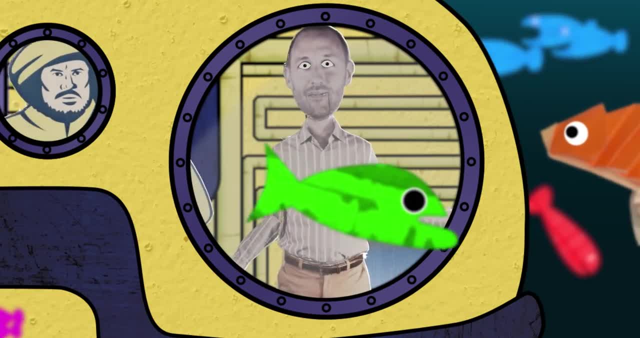 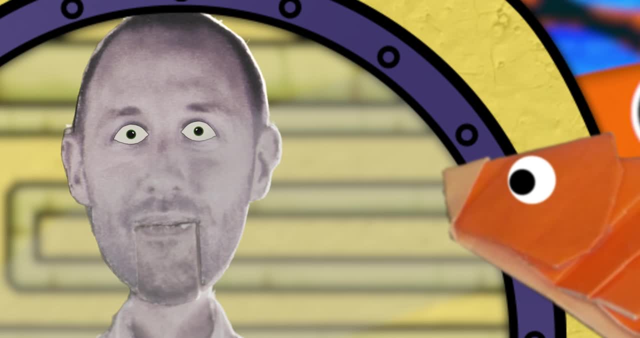 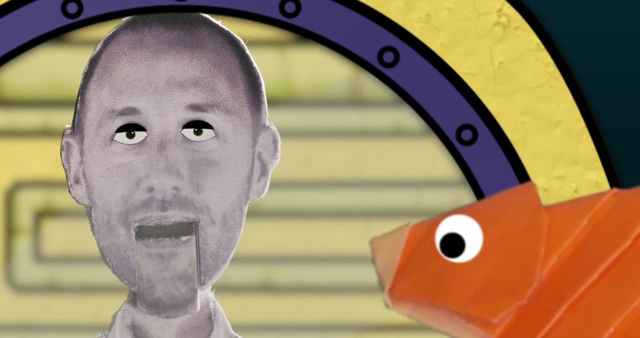 length of these fish is greater than the 35 centimeters, so we can start fishing. Let's get started. We'll begin with a question: Do we believe that the mean length of fish in this lake is truly greater than 35 centimeters, Or do we think our sample estimate of 41 ended? 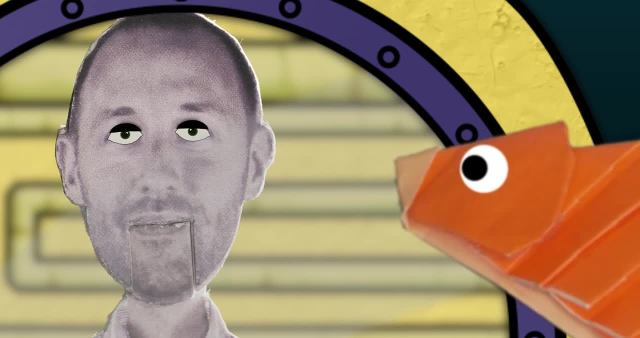 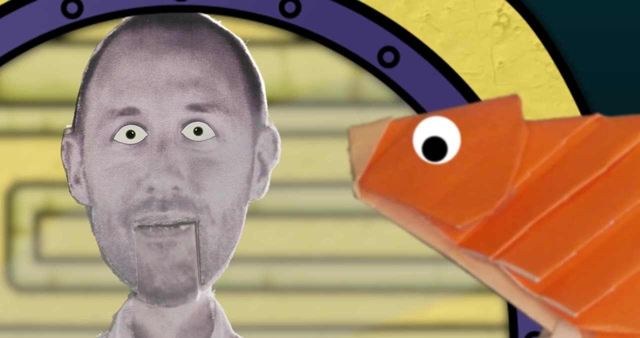 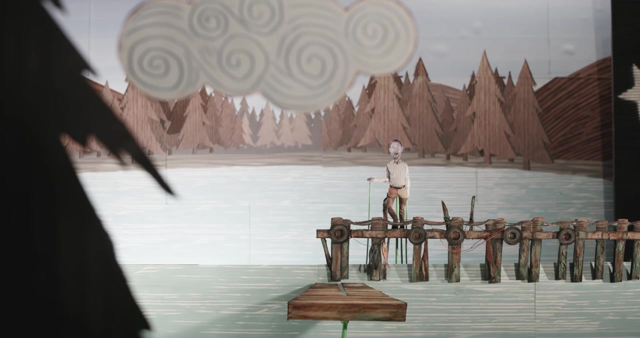 up being greater than 35 centimeters merely by chance. In other words, is there enough evidence to claim the true mean length really is greater than 35 centimeters? Man, oh man, do I hope so. To answer this question, we will begin by assuming that the mean length of fish in the 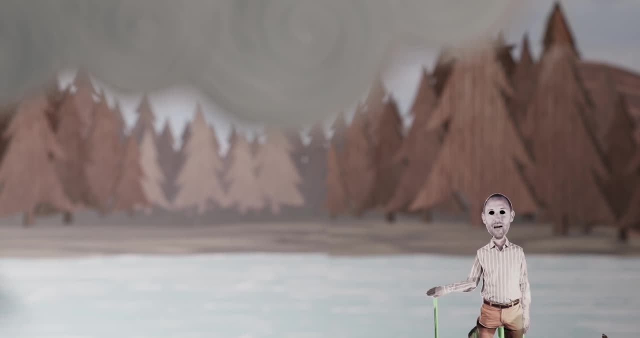 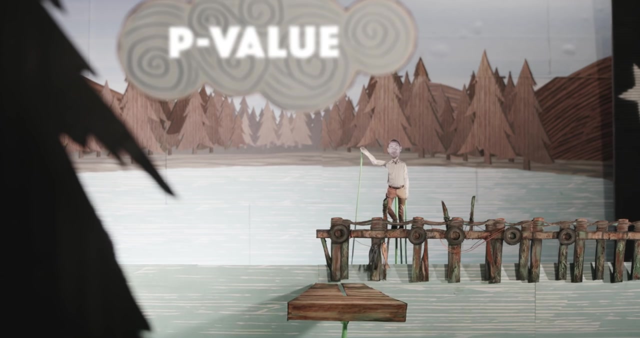 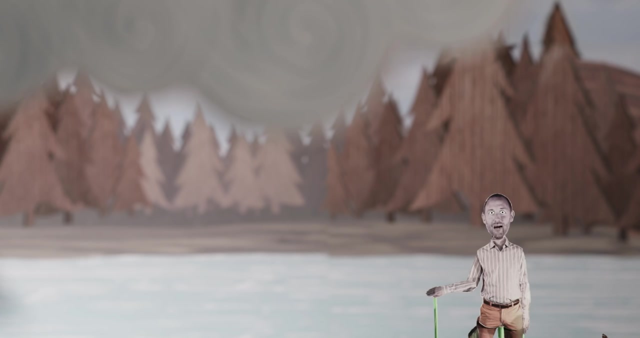 lake is 35 centimeters. The authorities won't let us fish unless the average length of fish is larger than 35 centimeters. From here we can calculate something called a p-value, which means that the mean length of fish in this lake is 35 centimeters. Now let's. 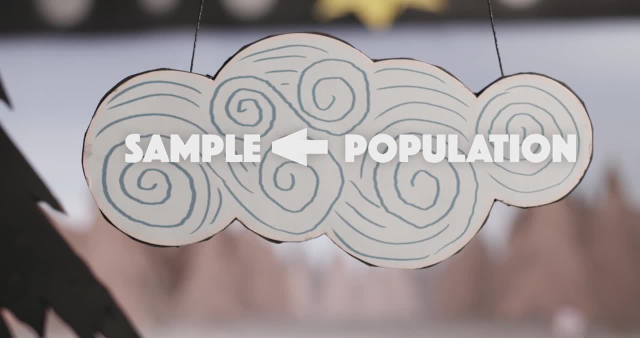 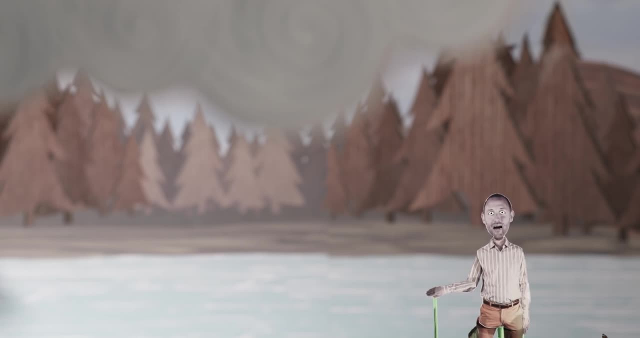 see how compatible our 41 centimeter sample estimate is with this assumed value of 35 centimeters. We would like to use our sample of 25 fish to try and make a statement about the population at large. Let's start with a hypothesis, or in other words, an assumption. 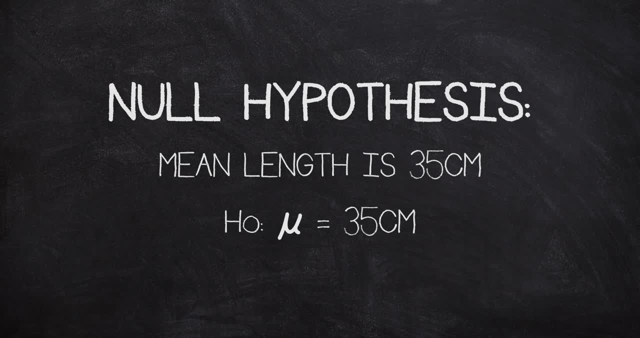 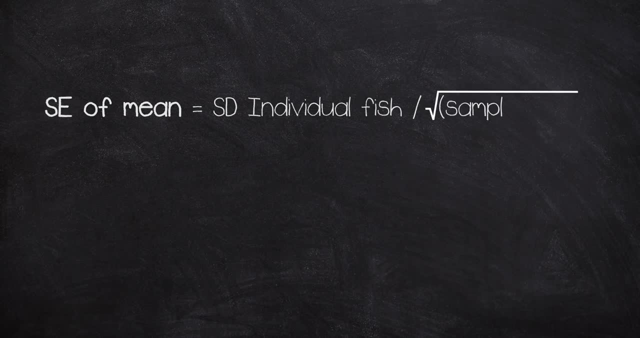 Let's assume that the true mean length of fish in this lake is 35 centimeters. This is what we call a null hypothesis. Man, oh man, do I hope so. The average length of fish in this lake is 35 centimeters. Since we don't know the true, 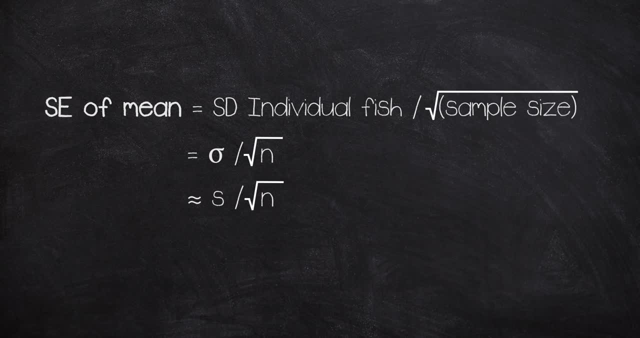 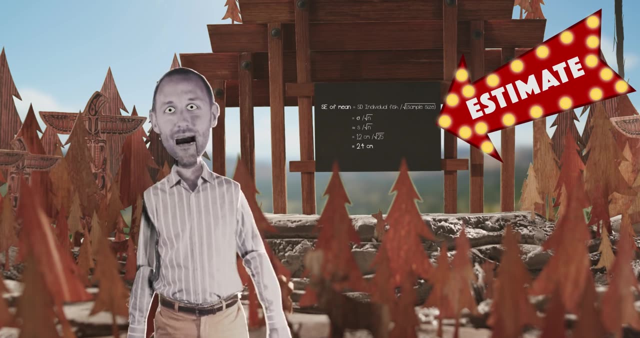 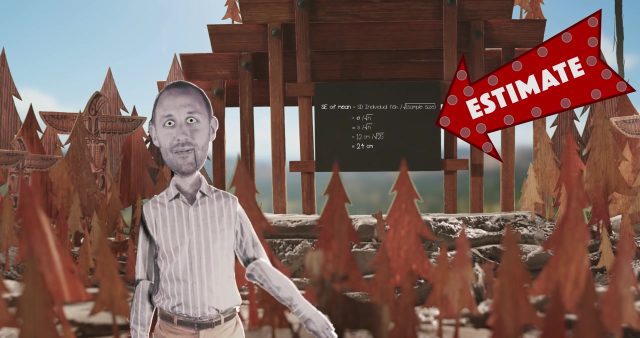 standard deviation we will substitute in the sample standard deviation in order to estimate the standard error of the mean. Recall that the standard error of the mean gives us an idea of typically how far a sample mean will deviate from the true mean. We would 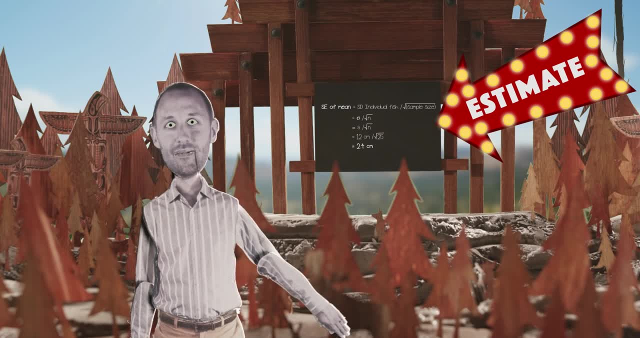 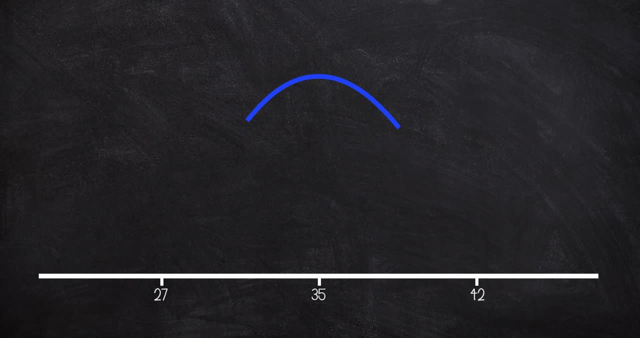 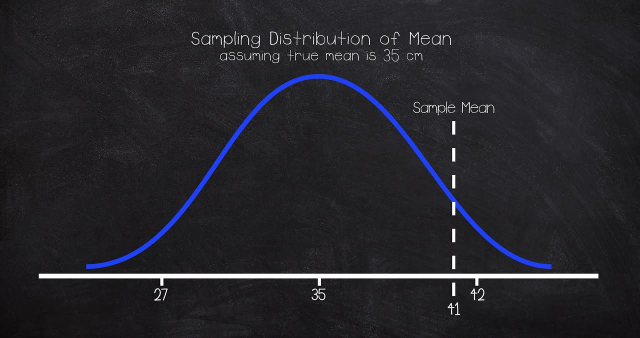 then know what the sampling distribution of the mean would look like under this null assumption that the true mean is 35 centimeters. Recall: we've taken a sample of 25 fish from the lake and found them to have a sample mean length of 41 centimeters. We can then ask the following question: Under our null hypothesis: 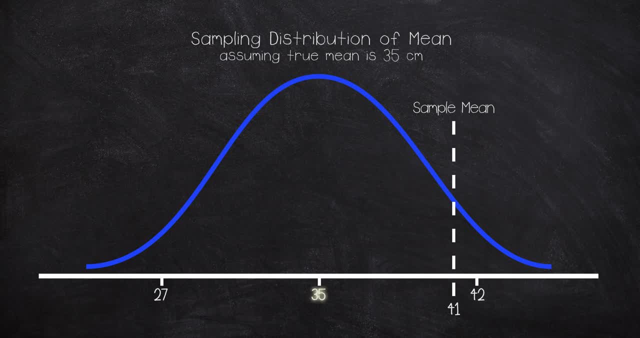 that the true population mean length of fish is 35 centimeters, what is the chance that we end up with a sample mean length of 41 centimeters or more? This probability is the p-value. If we were to calculate this probability, we would need to calculate the p-value of. 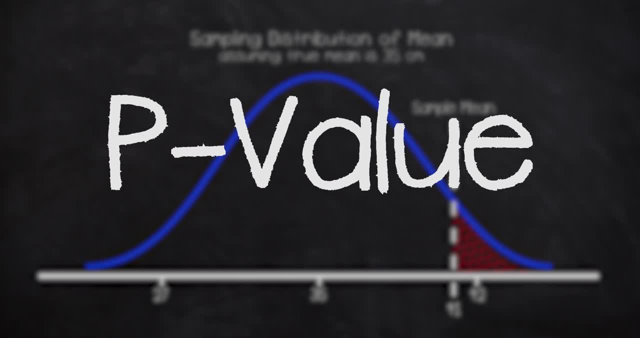 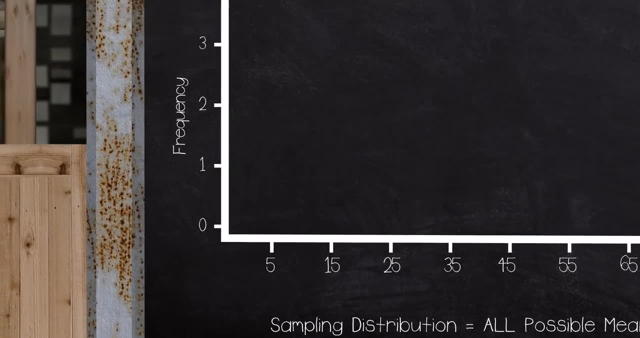 the fish. We would need to calculate the p-value of the fish. We would need to calculate the fish effect. We would find that it's approximately 1%, or one in a hundred Bye bye fish. In other words, if the true mean length really is 35 centimeters and we took 100 different. 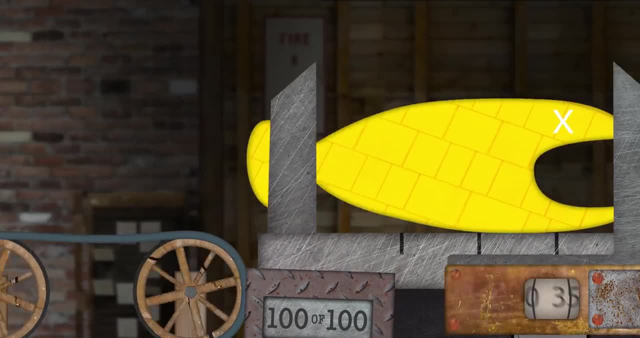 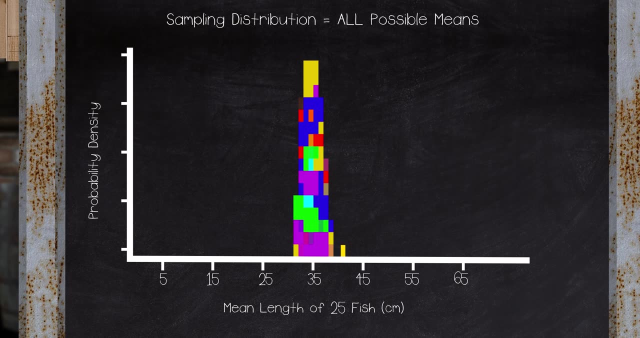 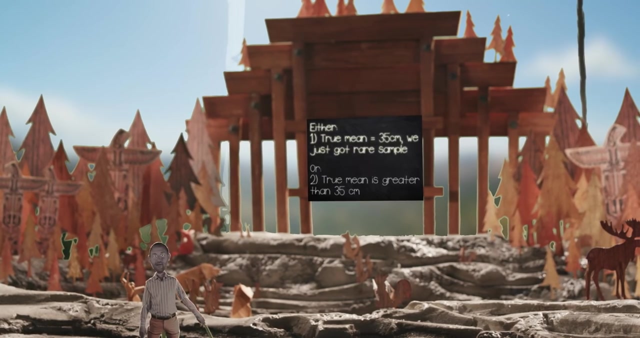 samples of 25 fish, we'd expect that only one of the 100 samples would give us an average length of 41 centimeters or more. by chance of theіл норм Bond S We can conclude that one of two things must have happened. Either our initial assumption, 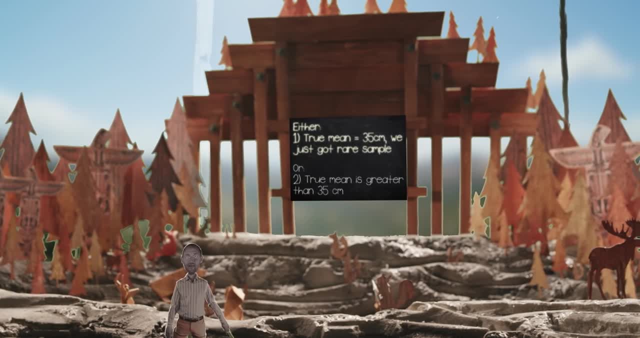 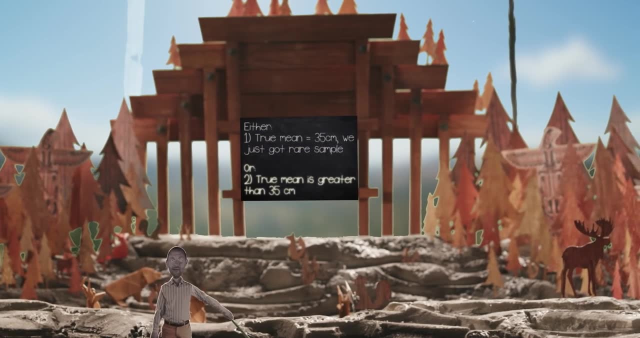 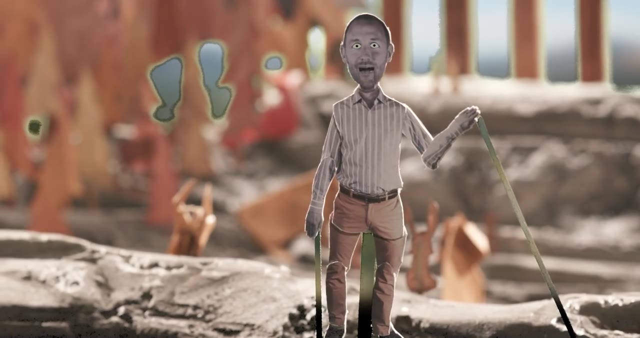 length is 35 centimeters is correct and we ended up with a fairly rare estimate of the sample mean- 41- just by chance, or our initial assumption is incorrect and the true population mean really is greater than 35 centimeters? we, of course, will never know for sure which of these is true in. 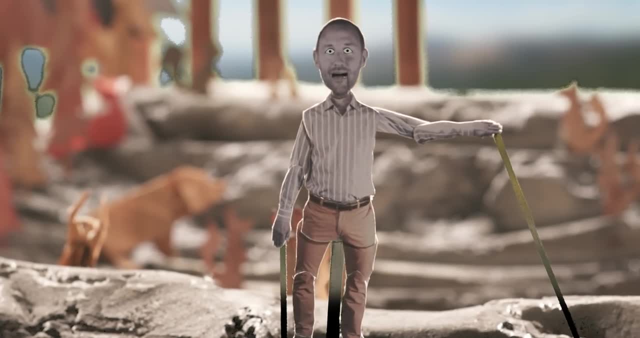 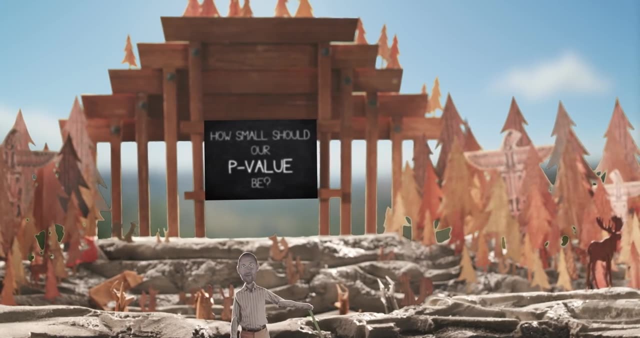 reality, but we can decide which we believe is more likely to be true. so how small should our p-value be before we will reject our null assumption? a general rule of thumb is to reject our null hypothesis if the p-value is less than five percent. and what's so special about that five? 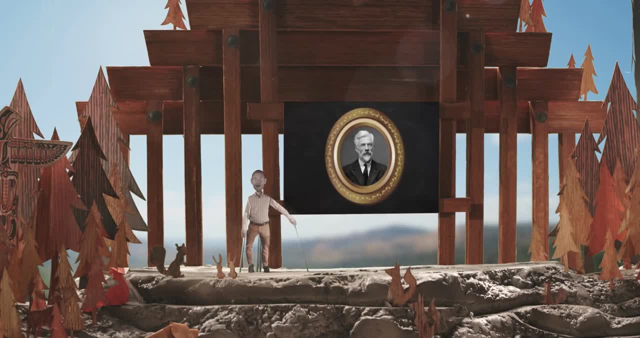 percent cutoff. you ask? it's because sir ronald fisher suggested this as a reasonable cut point and it stuck. it is a reasonable yet arbitrary choice. based on our p-value of one percent, we will reject our null hypothesis and conclude that we have enough and we have enough and we don't need to guard our hypothesis. it's a reasonable yet arbitrary choice. 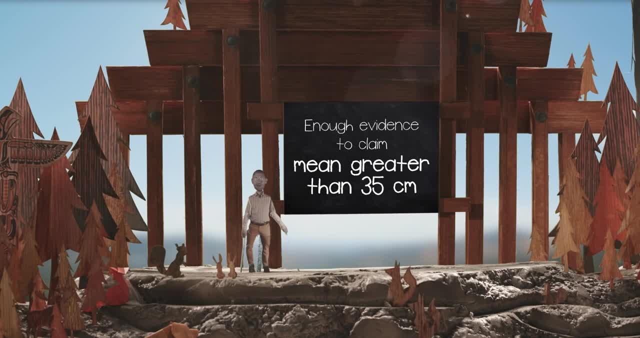 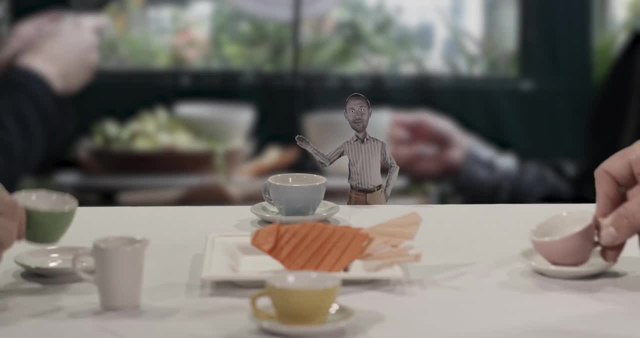 Based on our p-value of one percent, we will reject our null hypothesis and conclude that we have enough evidence to claim that the true mean length is greater than 35cm. Be careful: Relying solely on the p-value can be a dangerous thing, as it does not allow. 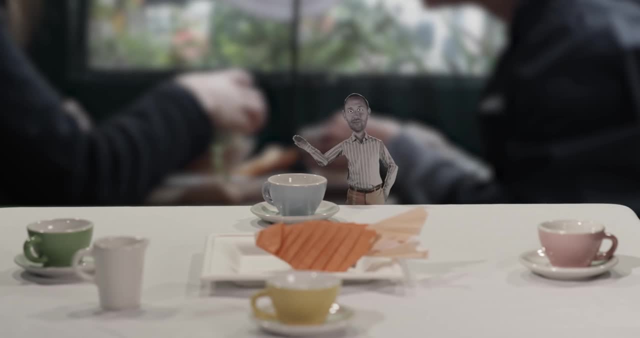 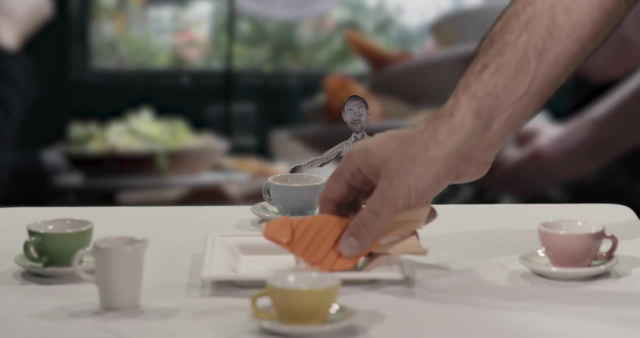 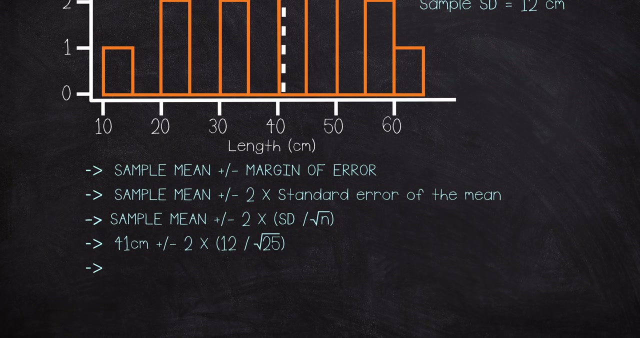 us to make any statements about the precision of our estimate. To strengthen our analysis, we should also construct a confidence interval for the mean. Previously we learned how to do this. We would say that we are approximately 95% confident that the true mean length of fish in this lake is between 36.2 to 45.8cm.